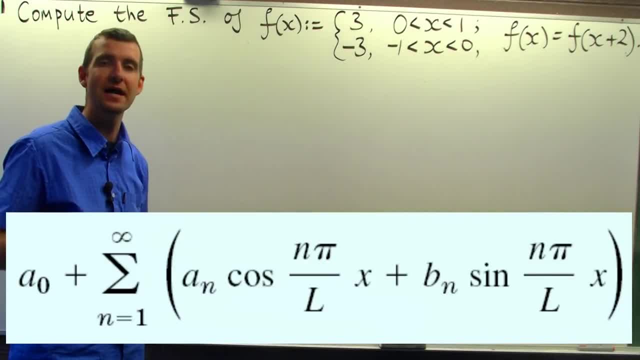 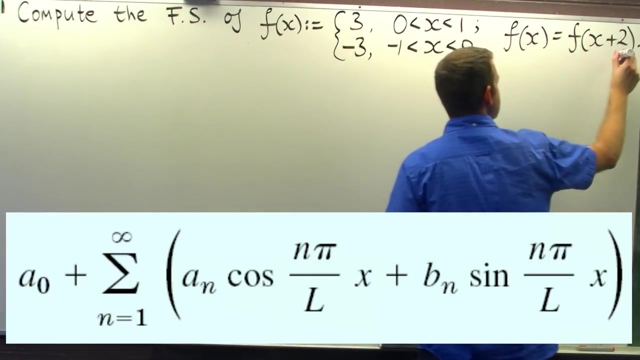 Well, Fourier series are an integral part of solving partial differential equations. These partial differential equations come from heat flow and, for example, the wave equation. Okay, but today's example is just simple: Calculate the Fourier series, and you do that by calculating the Fourier coefficients. Okay, so the first thing we note is that our 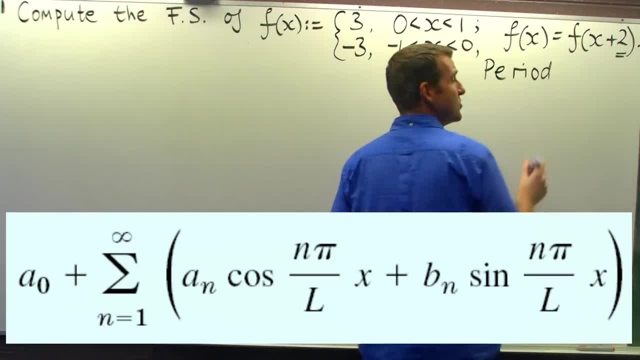 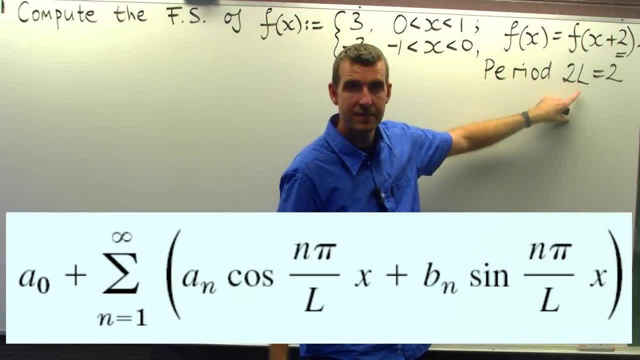 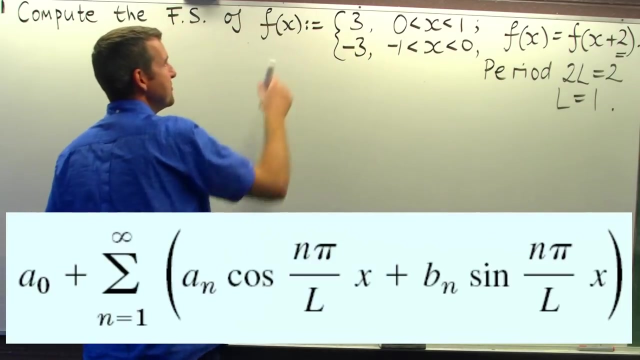 function has period 2.. All right now we write the period or denote the period by 2L. Okay, so in this case L equals 1.. This is important for finding our Fourier coefficients. Also note that the given function is odd. 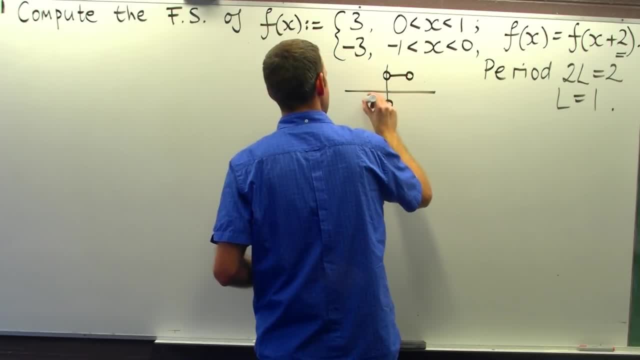 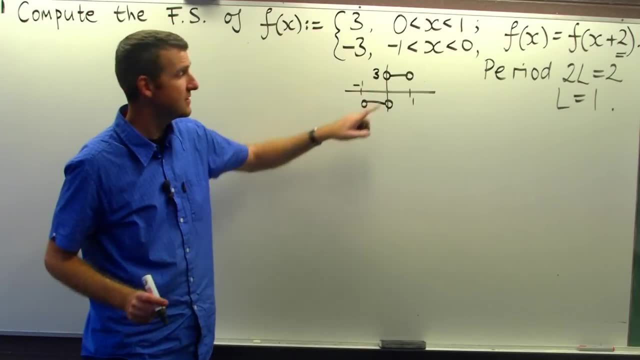 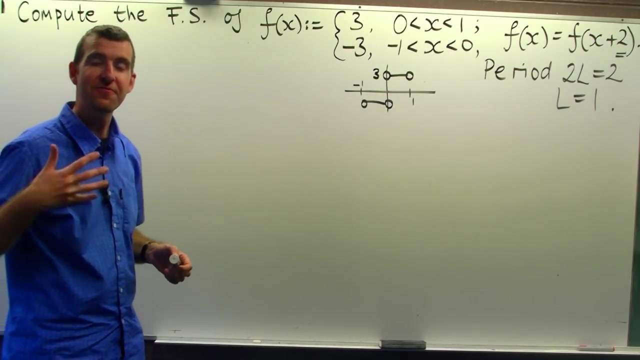 Okay. Okay, so this isn't drawn to scale, but the function is an odd function. Now, why is that important? Well, to compute the Fourier coefficients: the a naughts, the a? n's and the b? n's. 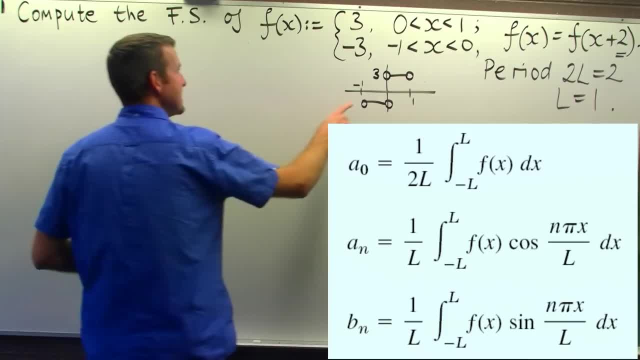 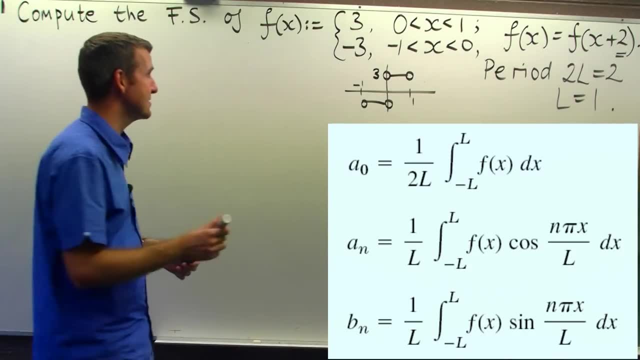 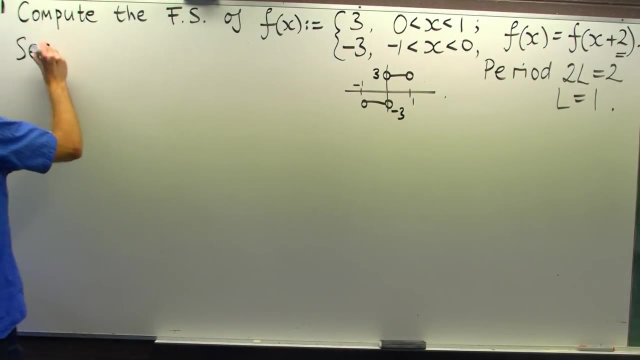 we rely on integration And we know that if we integrate, say, an odd function over the interval minus 1 to 1, things are going to simplify Okay. so it's very important. So the important observation is: f is odd. 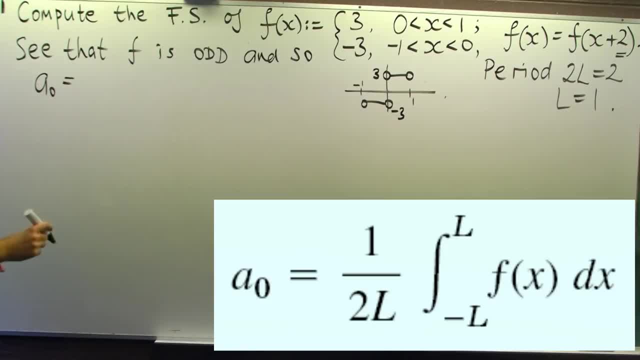 And so the a naught. if you look up the formula for a naught, it's just the following: So here I'm using the formula with big L equals to 1.. All right, well, we don't even really need to calculate this integral, because it's just. 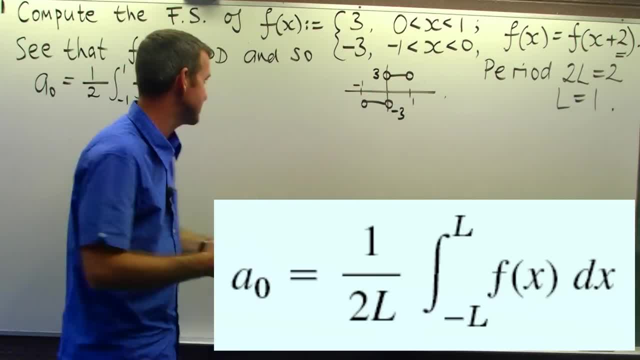 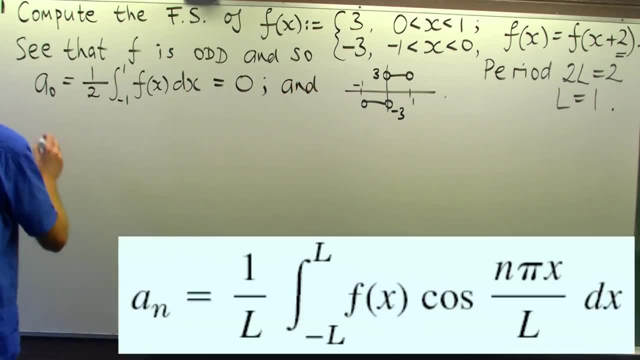 the area there which would be negative, And there they're just going to cancel each other out. We get 0.. Okay, What about a sub n for n greater than or equal to 1?? Well, applying the formula with big L equals 1,. 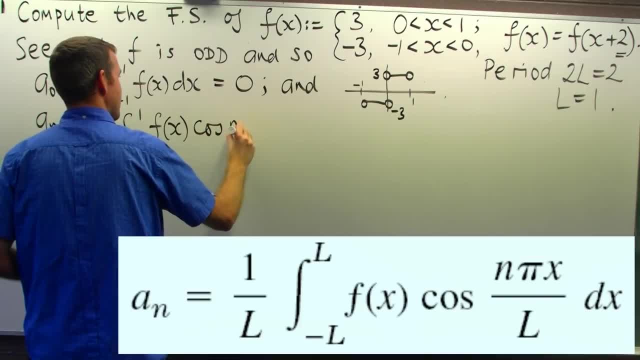 we want a square root of x equal to 1.. And then we're going to try to find out the function y, which is the small x. All right, well, we don't even really need to calculate this integral, because it's just the area there which will be negative. 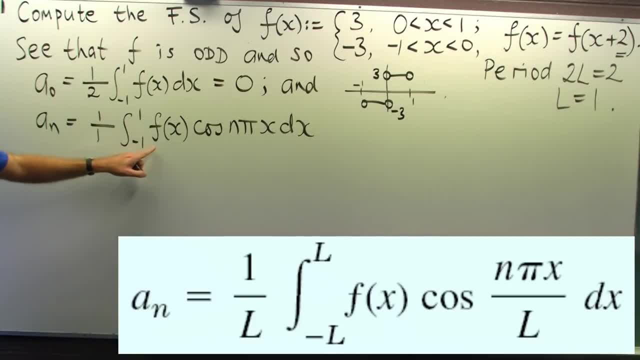 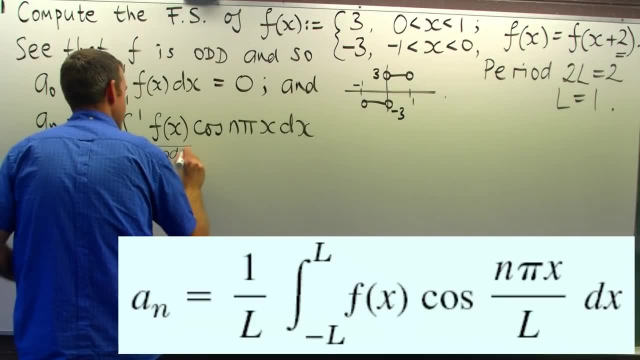 And there they're just going to cancel each other out to integrate this. But look closely: F's an odd function, Cos is an even function. So we've got the integral of an odd function times an even function, An odd function times. 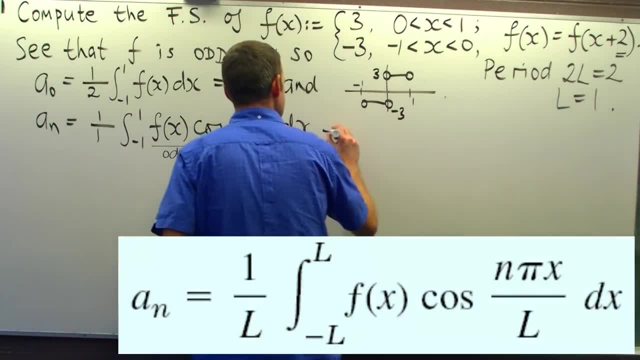 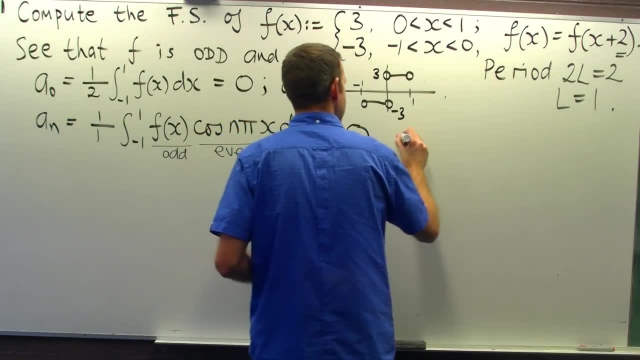 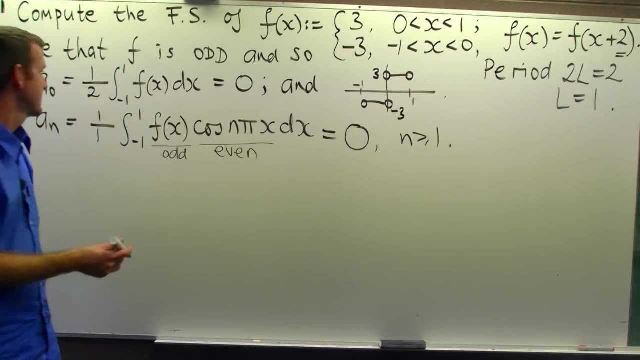 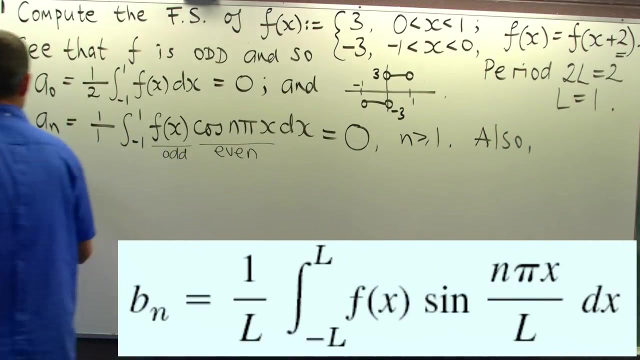 an even function gives us an odd function. So we're integrating an odd function between minus 1 and 1.. It's got to be 0.. Again, the areas cancel. So for each n greater than or equal to 0, this integral is 0.. Hmm, What about the b sub n? Well, b sub n is similar. 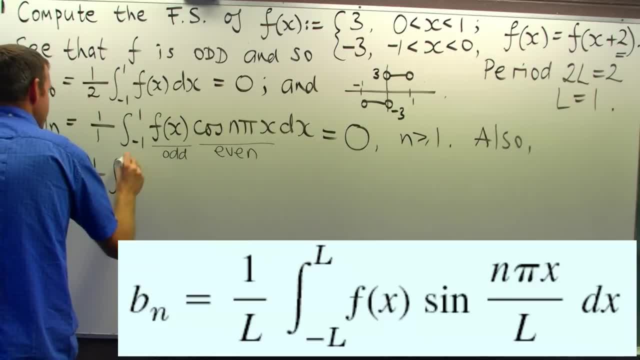 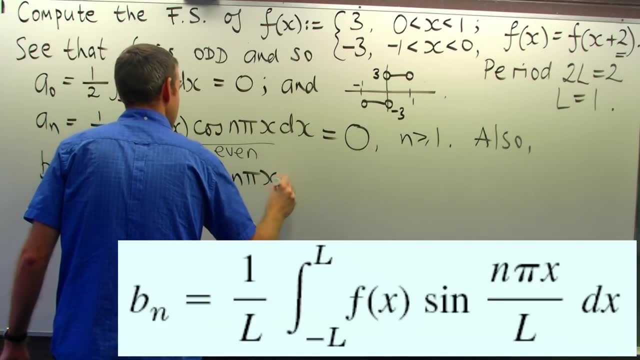 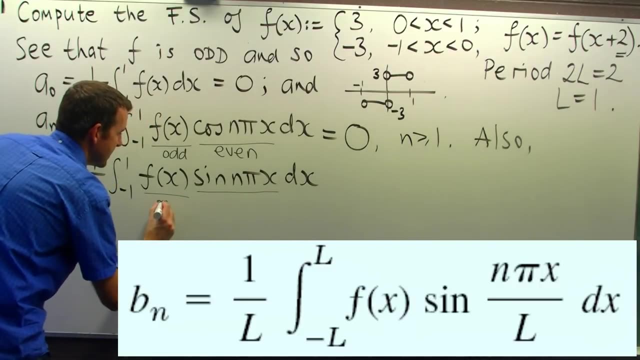 to this, but you replace cosine with sine, Alright. so where does that take us? Well, we've got an odd function, an odd function. The product is an even function. Now, if we integrate an even function between, say, minus, 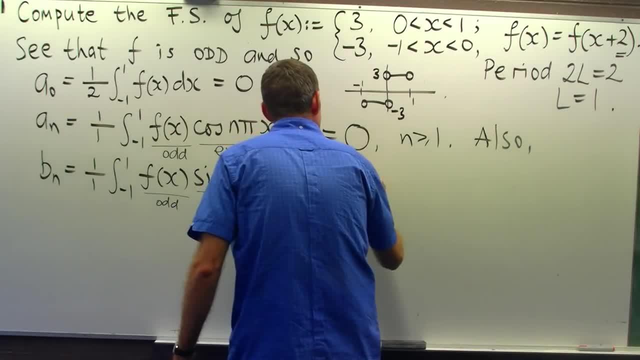 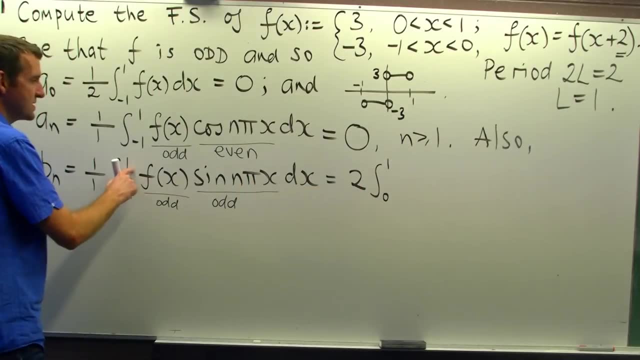 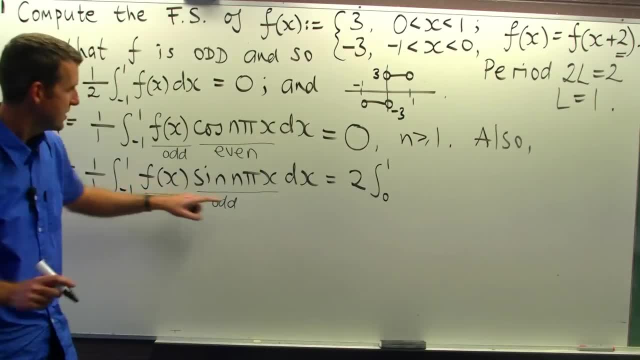 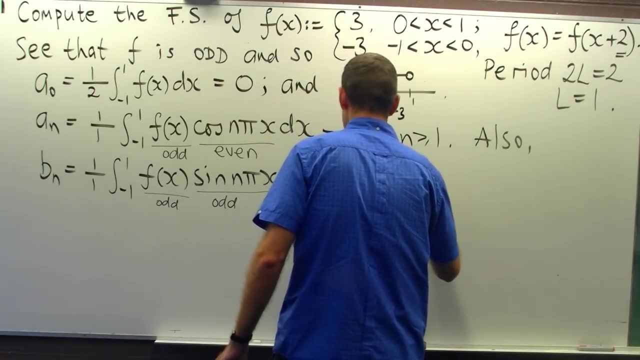 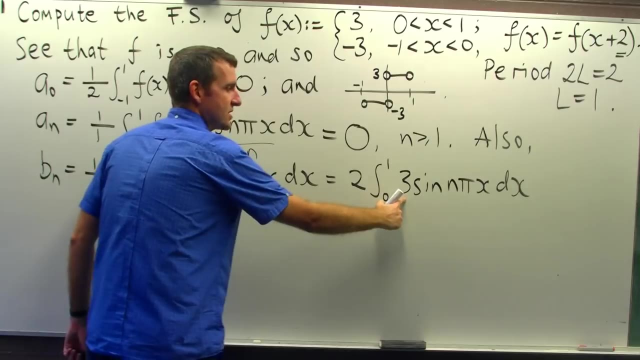 minus 1 to minus 1 to minus 1 to minus 1.. Okay, so, on this interval 0 to 1, f of x is 3.. So we replace f of x with 3, sine n, pi, x, dx. Now 3 is just a constant, so I can. 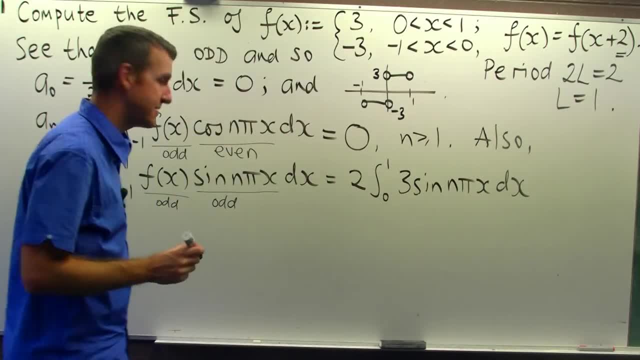 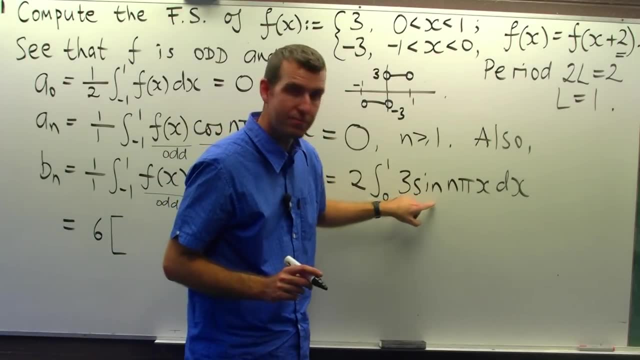 take it out the front and I want to integrate sine n pi x. So let's do that, So I'll get 6 out the front. When I integrate sine, I get minus cosine and I've got to divide by n pi. 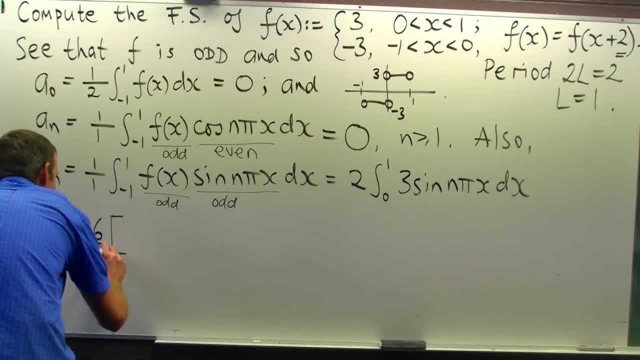 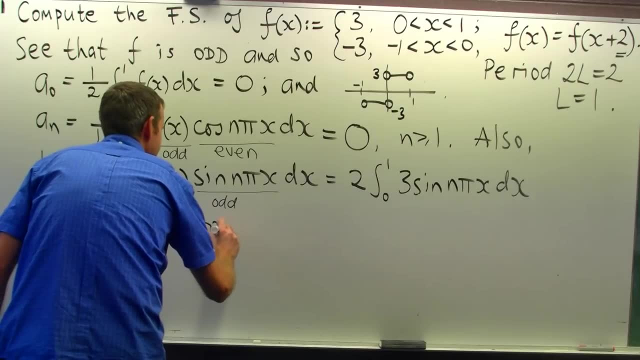 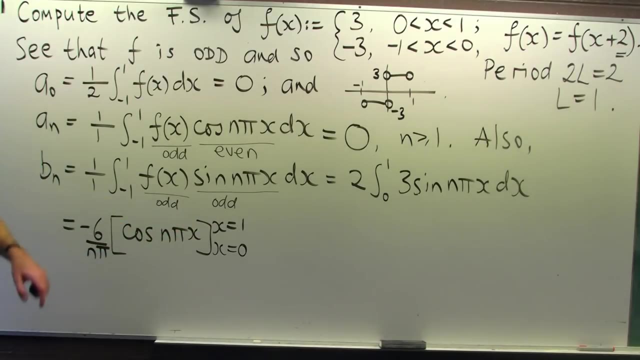 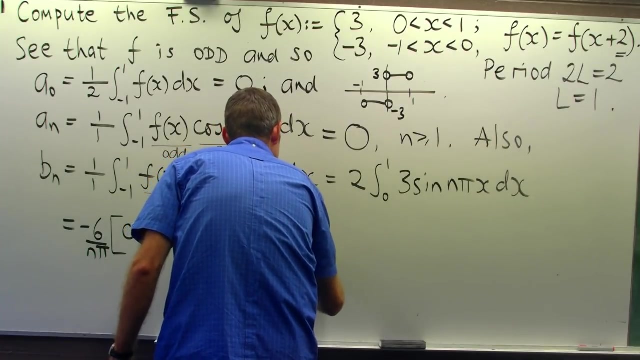 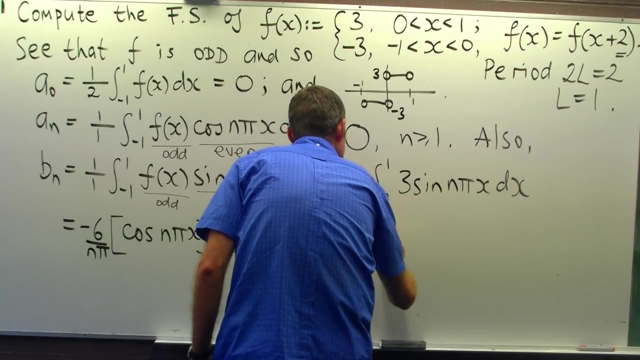 So I'm going to bring that minus out, the front divide by n? pi, and I'm going to get cos n pi x. All right, So now it's time to put in x equals 1 and x equals 0.. So here I'll get cos n pi minus cos of 0, which is just 1.. 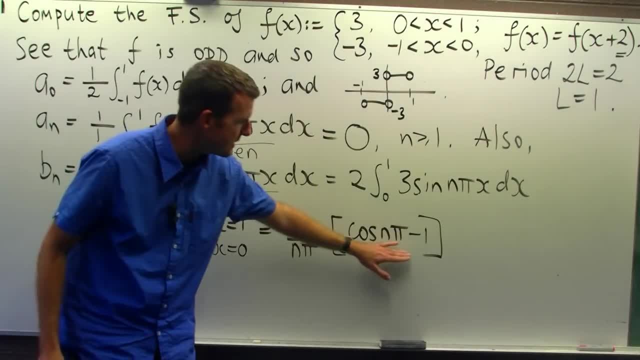 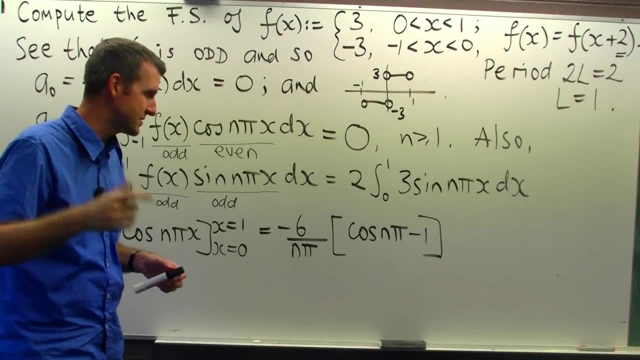 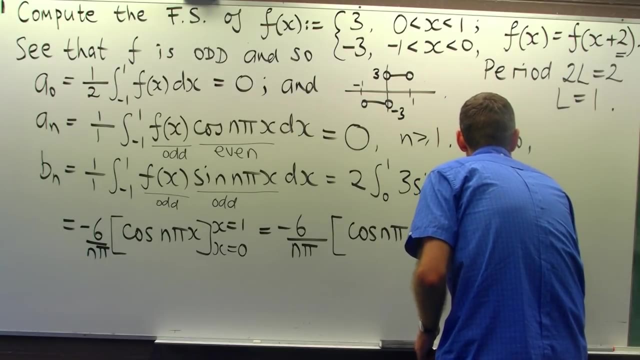 Okay. so what do we do now? Well, we can clean this up a bit. Cos n pi. it goes: positive 1, negative 1, positive 1, negative 1.. So cos n pi is actually the following: You can write it in the following way: 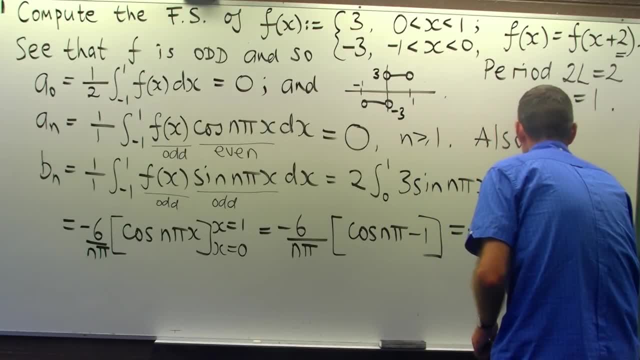 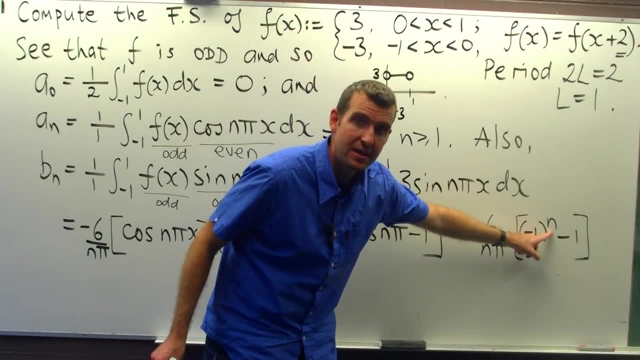 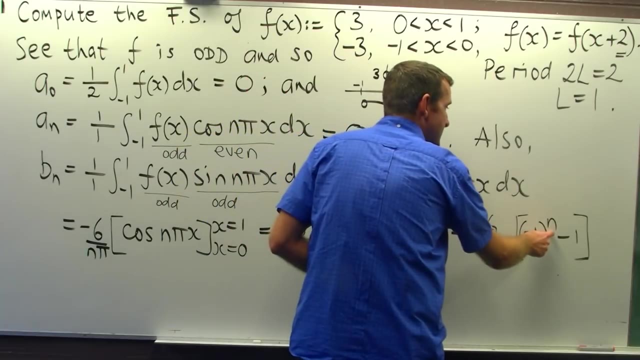 It's an oscillating sequence. Okay, We can still go a little bit further here. If n's even, this is going to be 1 minus 1, so it's 0.. If n is odd, then this is going to be minus 1, minus 1.. 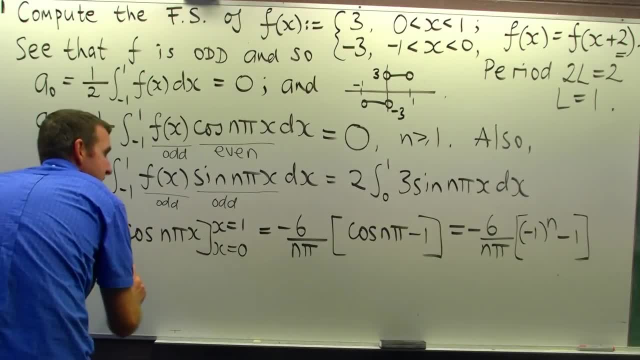 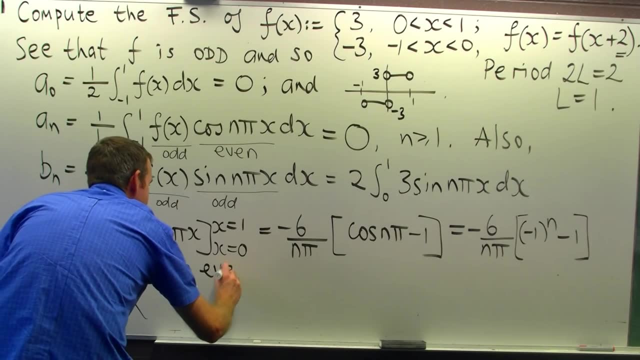 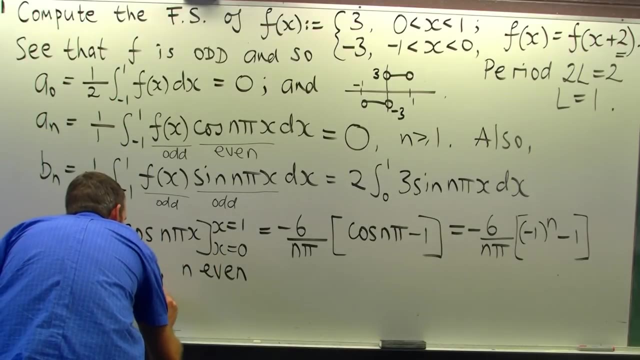 So we can go a little bit further and it's going to be this: 0 for n even, and if n's odd, we get minus 2 here, Minus 2 times minus 6 on n pi, 12 on n pi when n is odd. 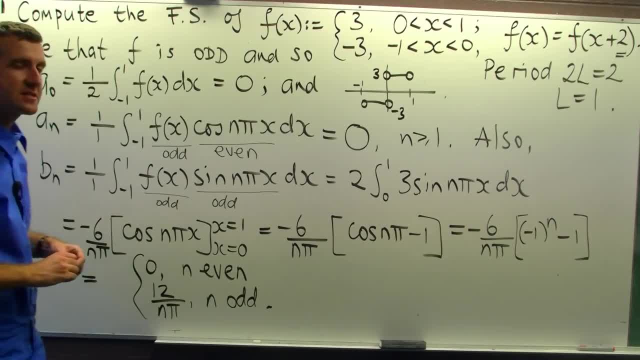 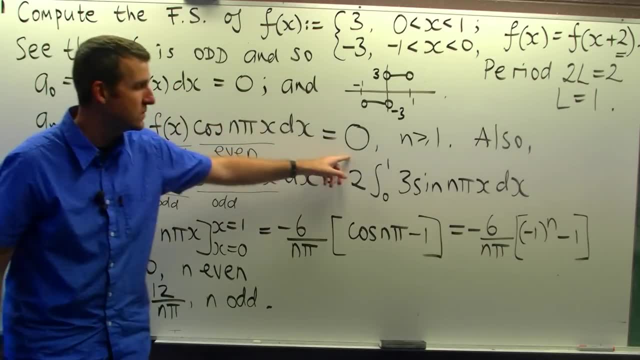 Okay, So what's our Fourier series? Well, let's go back to the formula for Fourier series. Now a naught 0.. The a? n's are all 0.. The b? n's, well, they're 0 for n even. 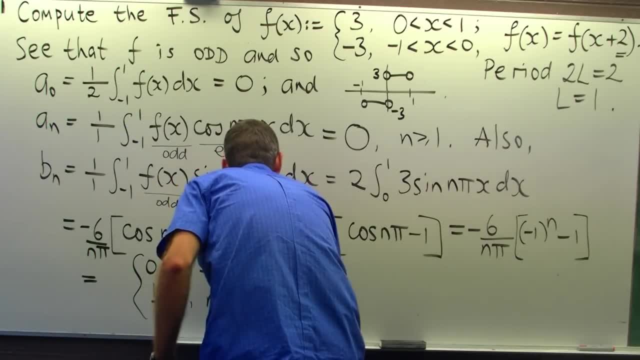 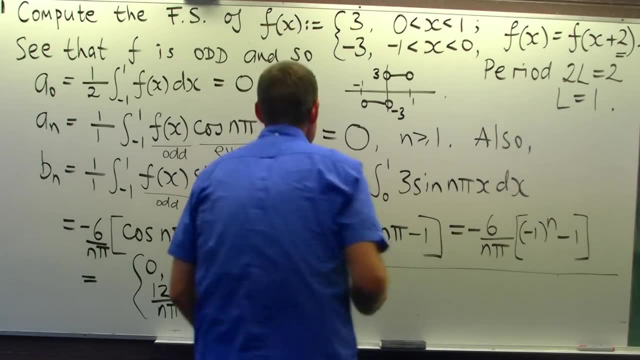 and 12 on n pi. So let's write out our Fourier series. Now I denote the Fourier series of little f of x by big S f of x. So a naught 0,. a n's are 0, and it's the only non-zero ones. a, b, n for n- odd. 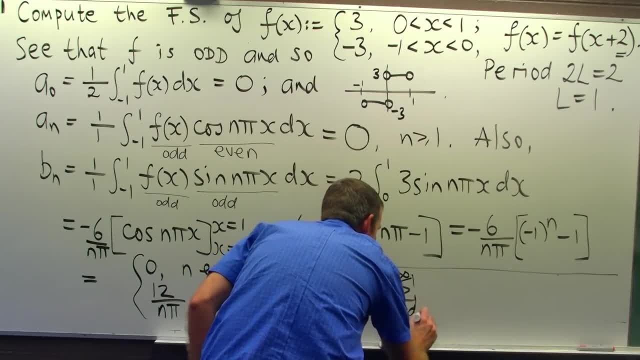 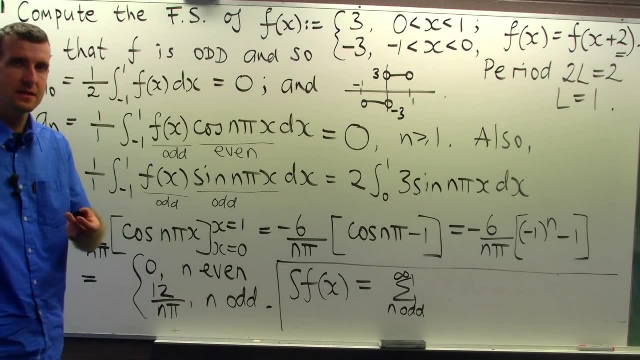 So look what I do here: I'm only adding. well, I'm only putting in those n that are odd In the sum, Because otherwise, if n's even, then I'm not. I'm just adding 0. 0 together, right.